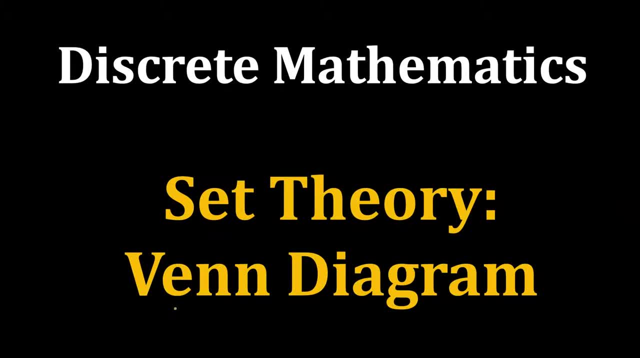 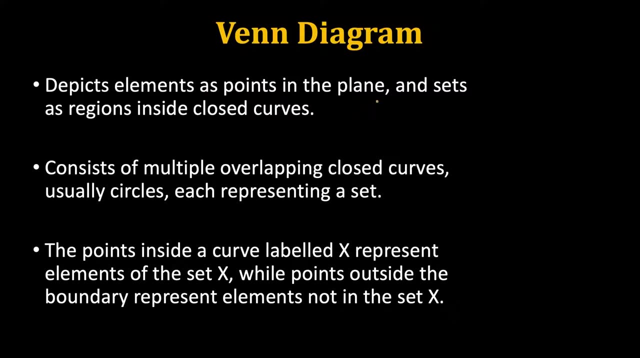 In this video we are going to see an interesting way of representing the sets and it's very intuitive and easy to understand the concepts, and this is called Venn diagram. So in Venn diagram, elements are represented as points in a plane and the sets are represented as closed regions, regions enclosing those. 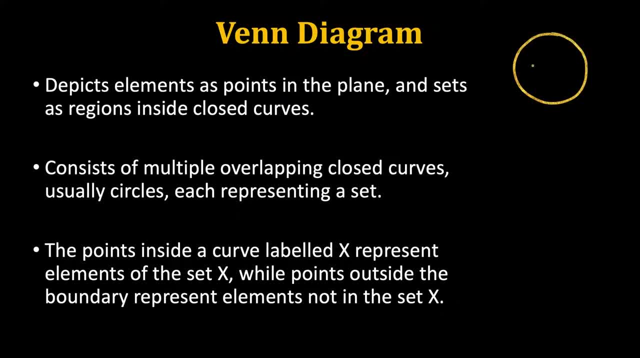 points. So this is a set. so usually we denote this by circles, these closed curves, and inside we have the elements of the set. So this is a set, let's say X, and these are the elements of the set. So let's see some concrete example then it. 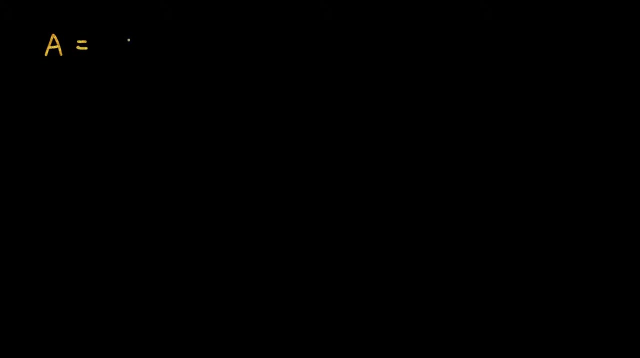 will be more clear. Let's say we have two sets, 1,, 2, 3, then set B, which consists of 5,, 6, 7. Then, if we have to represent this as Venn diagram, we will draw two. 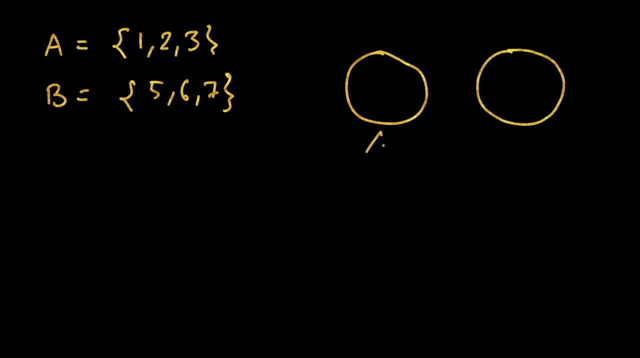 circles corresponding to two sets. then A has 1,, 2, and 3, and b has 5,, 6, and 7, and there is no element common to these two sets. so these two circles are connected Now and we usually denote everything inside a rectangular region which we call. 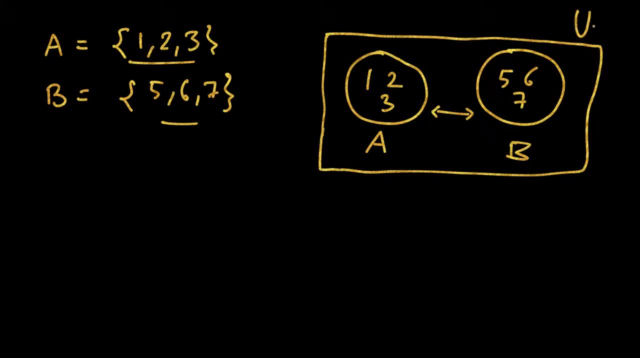 this universal set and we denote it by U. So in a given context, the elements of the set can take only fixed value and all the possible values, the union of all those possible values we call the universal set. Now let's take another example, and this time we will. 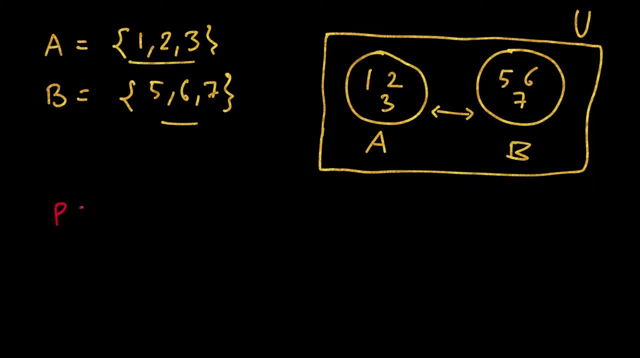 have some common elements. Let's say we have one set, P is equal to 1,2,3,4, and set Q has 3,4, 8,9.. So we see that 3,4 is common to both of these. So we will First draw P and